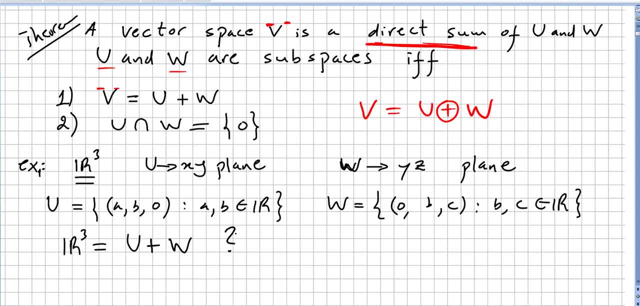 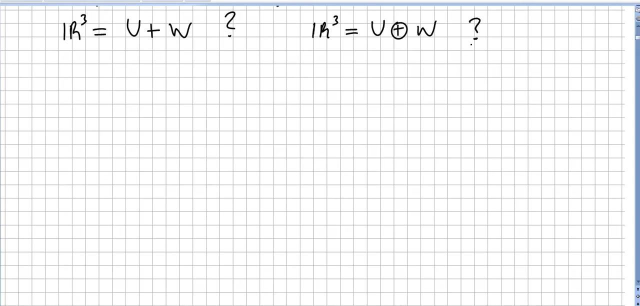 question? well, yes, because every vector in r3 is the sum of a vector in u and a vector in w. okay, that's easy to to prove. now the question is: is r3 equal to the direct sum of subspaces u and w? so let us see if this is true. so this one is true. right, i can erase this one. 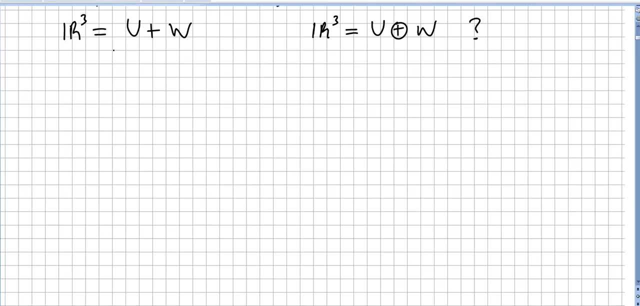 because we can, this is true. we can easily uh take the, the addition of these two subspaces. now, what about the direct sum? okay, uh, let us pick one vector in r3, let us say three, five, seven, and we can see that we can write this vector as: 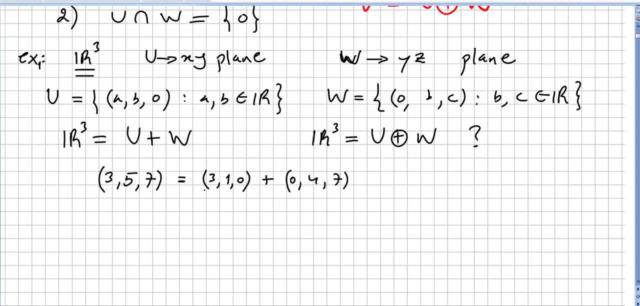 we can write three, five, seven as the addition of three, one zero plus zero, four, seven, right. three plus zero that will be three, one plus four that will be five, and zero plus seven that will be seven. okay, but i can also write these vectors: three, five, seven as the addition of three minus. 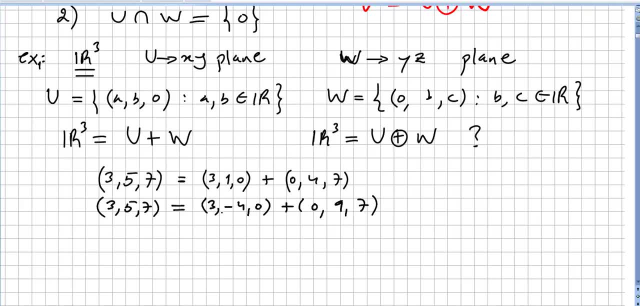 four, zero and zero, nine, seven. right, three plus zero, we get 3 minus 4 plus 9, that's 5, and 0 plus 7, that's 7.. so we have two ways of getting this vector as an addition of u, subspaces u and w. so there is not a unique way of every single vector in r3 or in r3. 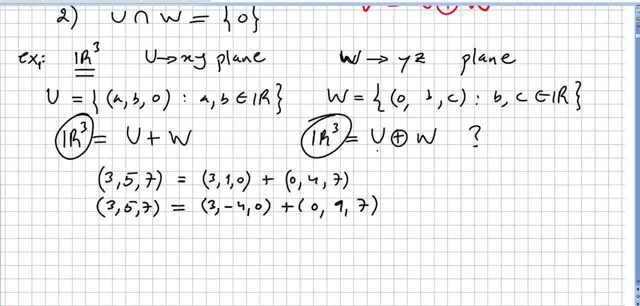 there's not a unique way of writing this as sum of those two, okay, of the vectors in those two subspaces. so that would be my first argument. and second, we have vector 0, 1 0, 0 1 0 will be a vector in the.